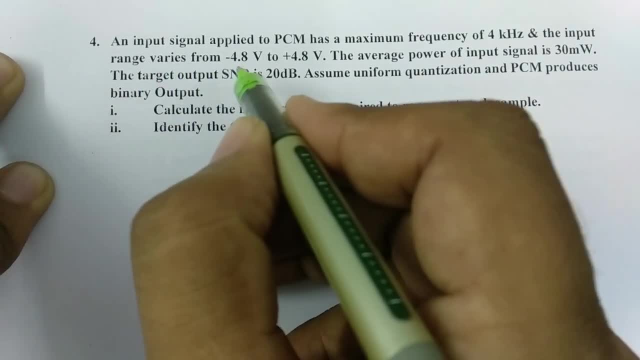 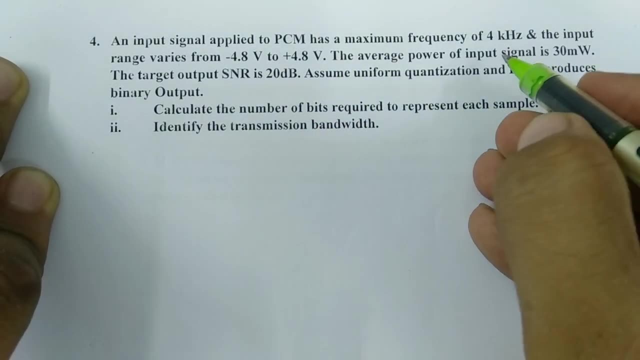 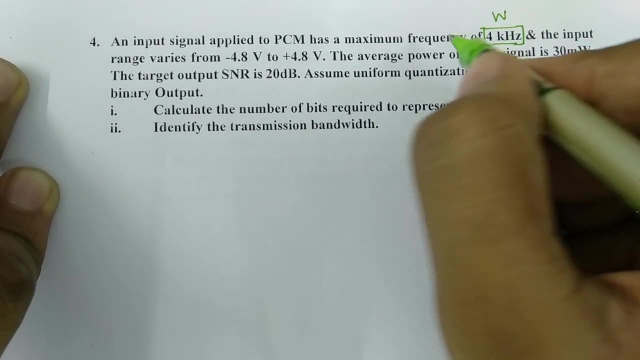 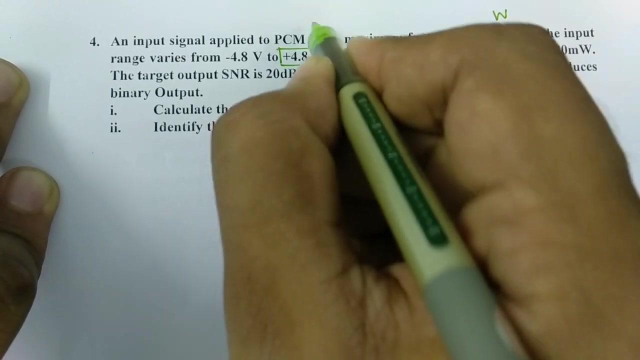 4 kilohertz and input range varies from minus 4.8 voltage to plus 4.8 voltage. So here one thing that is here like see. maximum frequency is 4 kilohertz means bandwidth of signal that is 4 kilohertz, and input voltage ranges from minus 4.8 voltage to 4.8 voltage means maximum voltage. that is given by 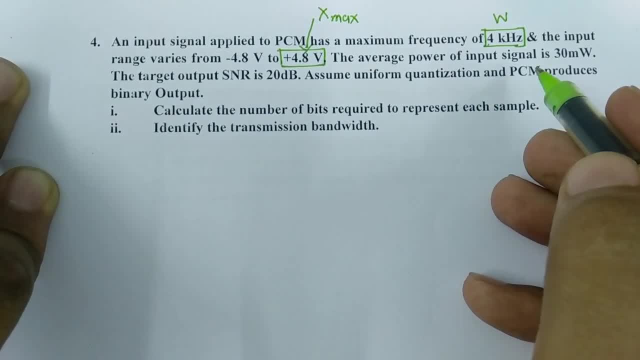 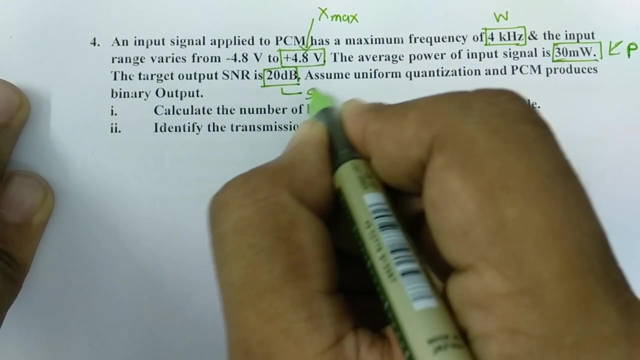 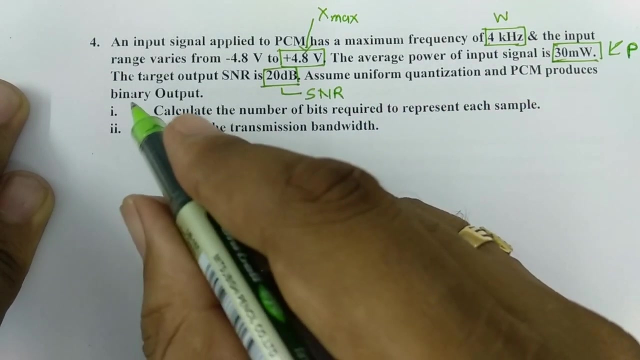 4.8 voltage. The average power of input signal that is even given that is 30 millivoltage. So power that is given by 30 millivoltage and target SNR that is even given 20 dB. So target SNR that is even given 20 dB. Assume uniform quantization and PCM produce binary output. Calculate the number of bits required to reply to PCM. 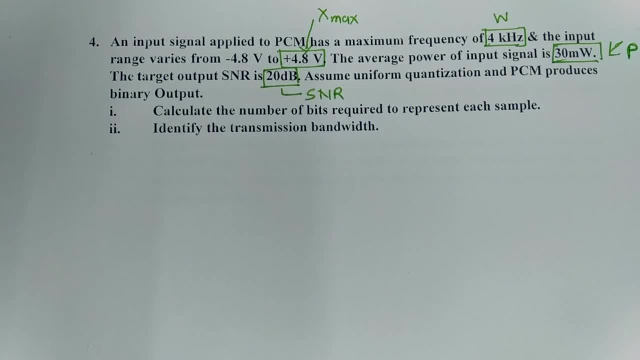 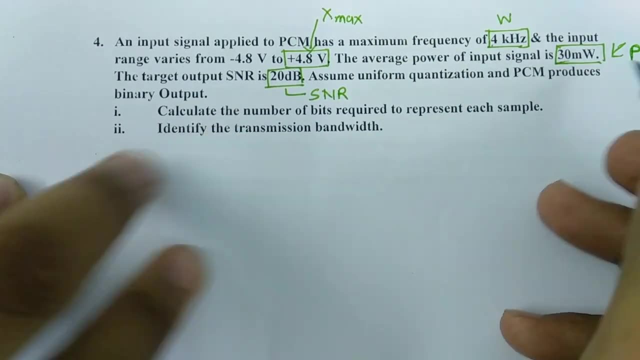 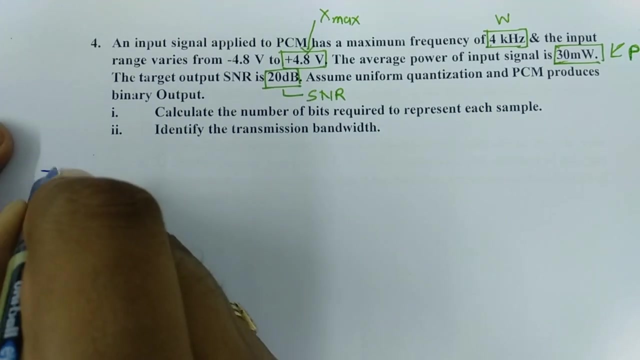 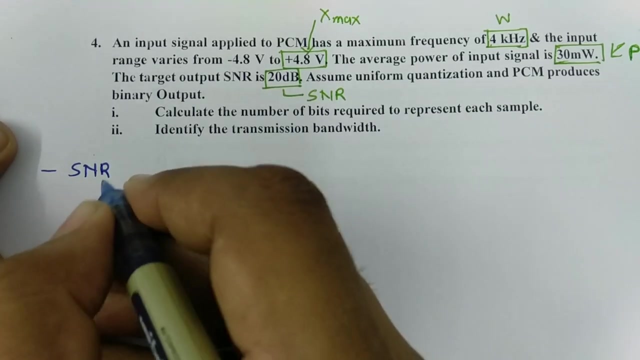 Present each sample and identify transmission bandwidth. So here see maximum amplitude, bandwidth as well as power is given and SNR is given. So if input signal is not sinusoidal, in that case we need to use this formula of SNR, SNR. and now this SNR is not there in terms of dB, it is there in terms of magnitude. So magnitude, SNR, that will be 3.5. 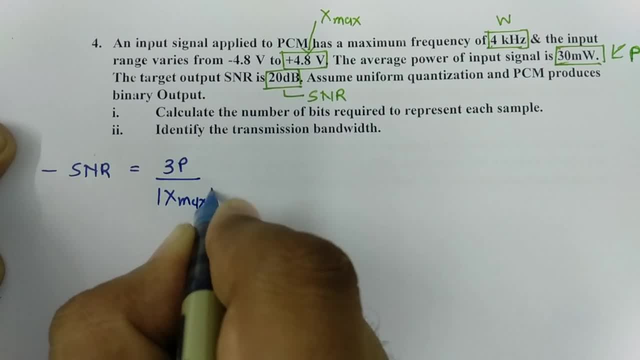 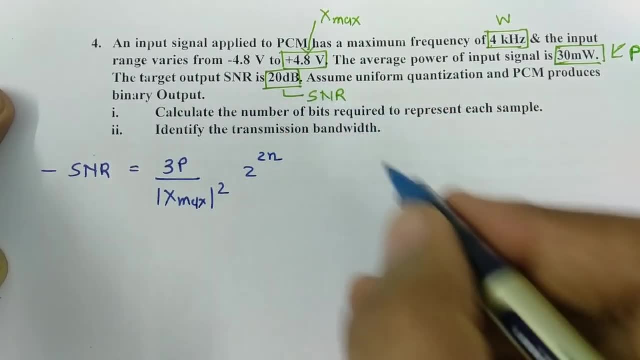 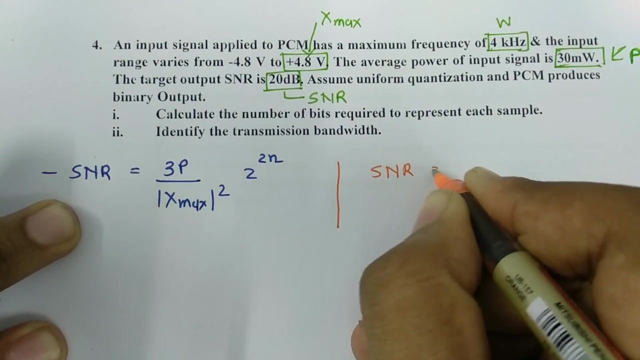 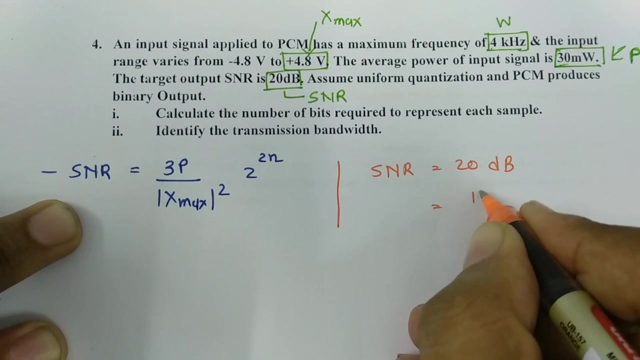 We have CP divided by maximum amplitude, squared into 2 to the power twice n. So this is what the basic formula Now see: here SNR is 20 dB, Here SNR is 20 dB. So if SNR that is 20 dB, it means in terms of magnitude you will be getting, it will be 10, it will be anti log of this. So 10 to the power of 2, it will be the peak. 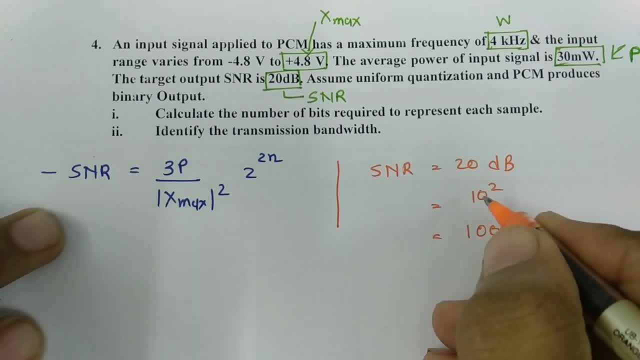 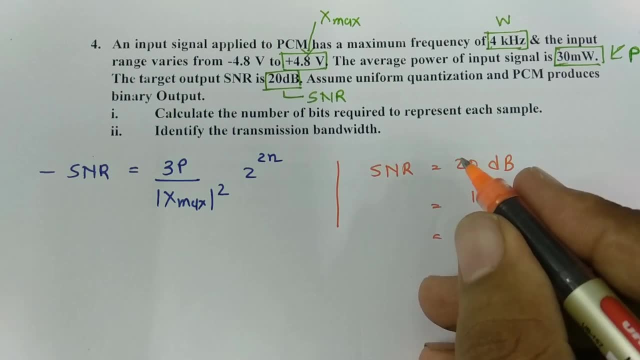 that and you will be getting it is 100. so when you have this snr in terms of db, calculate that in terms of magnitude. so you just do 20 divided by 10 and antilog of that. so if you do that then you will be getting it will be 10 to the power 2 and that will be 100. so in terms of magnitude, 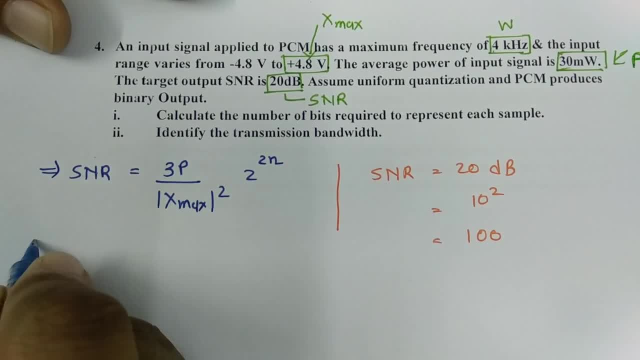 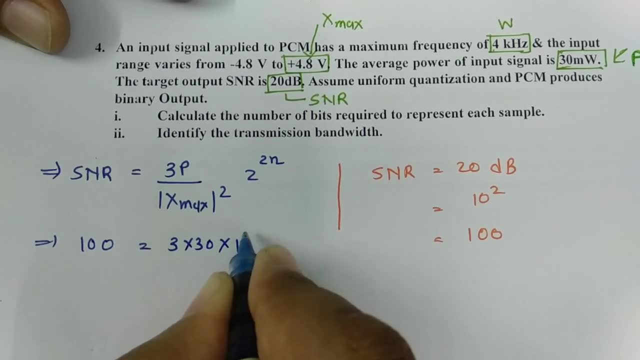 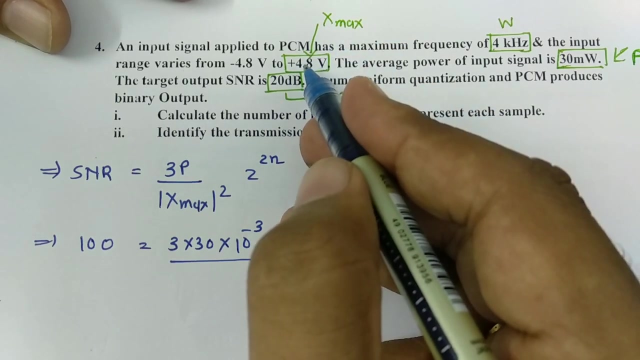 snr is 100 and now just place that so 100 power is 30 milli voltage. so 3 into 30 milli means 10 to the power minus 3 into 1 divided by x max, square x max is actually 4.8 voltage. 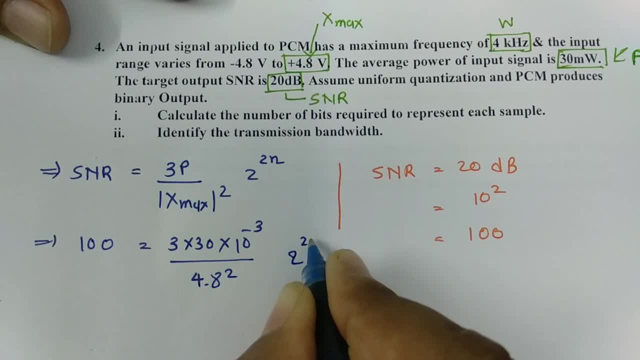 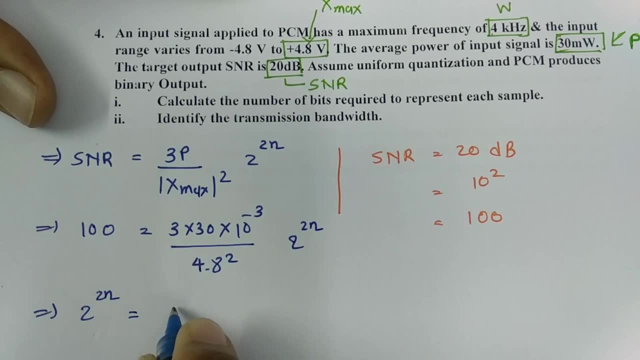 so 4.8 square into 2 to the power twice n. so now here we'll be calculating 2 to the power, 2 n, that is equals to 100 into 4.8, square divided by 3. divided by 30, 10 to the power minus 3 into 1 divided by x max square x max is actually 4.8 voltage. 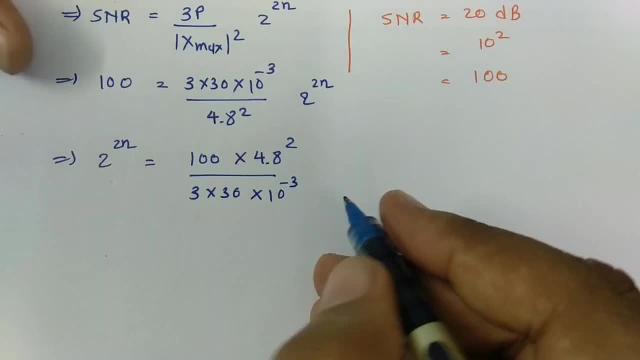 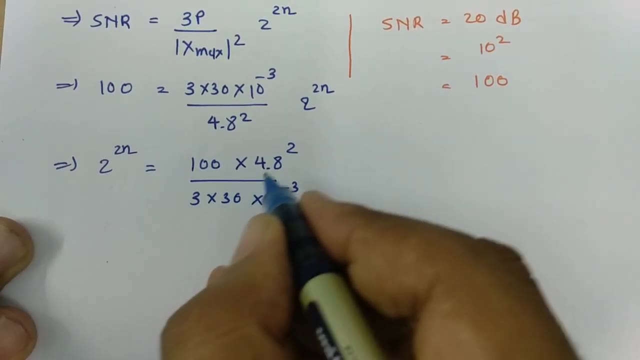 so that's 2 to the power minus 3, that will be 2 to the power 2, n, and if you calculate this you will be getting n value. so you just do this calculation. all you need to do is you just calculate this value and then take log at both of the side. and if you take log both of the side, 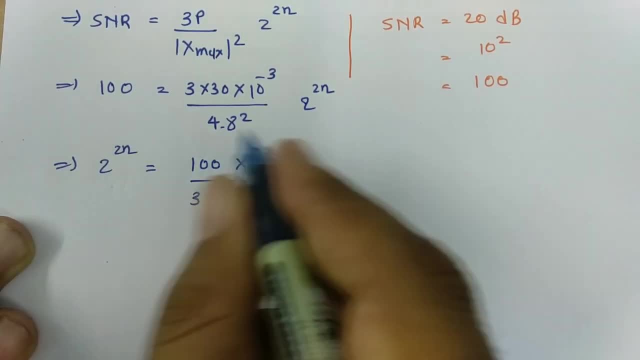 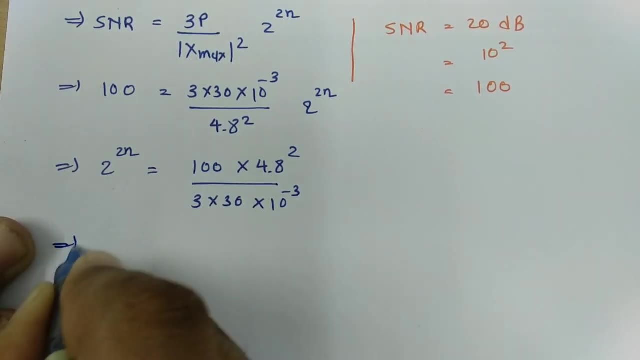 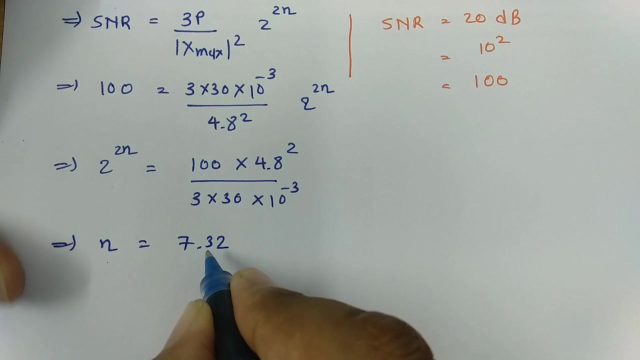 you will be getting 2 n over here and divide by log 2 of this log 10 base, so that division will result into 2 n and you will be getting n, so that n you will be getting by 7.32. now see 7.32. that is what exact answer, but bits cannot be taken in. 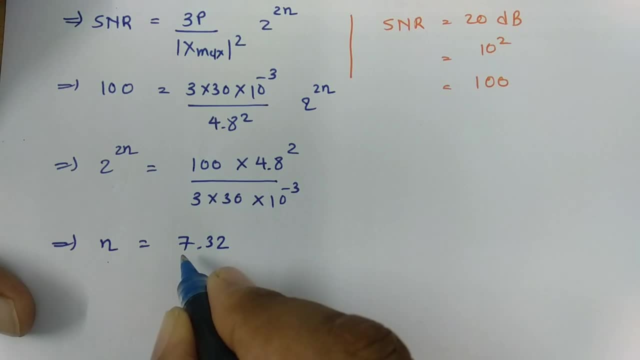 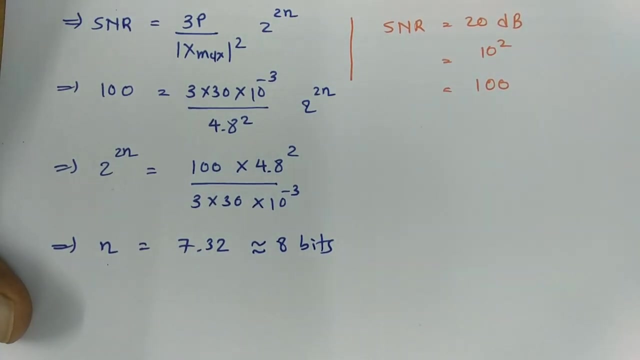 terms of fractional values. so you have to take round off here at larger value. so it will be 8 bits. so 8 bits that is required to represent this pcm pulse code modulation. now here a transmission bandwidth. that is the second question. now, as we know, transmission, 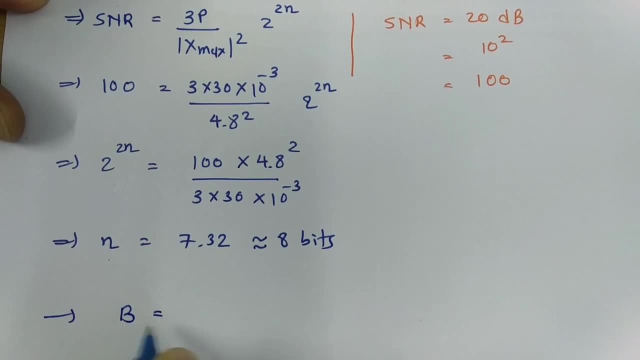 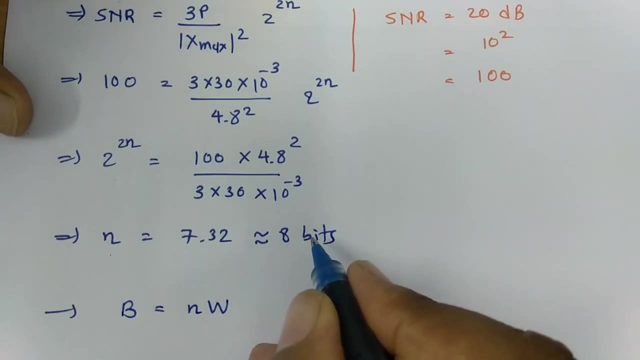 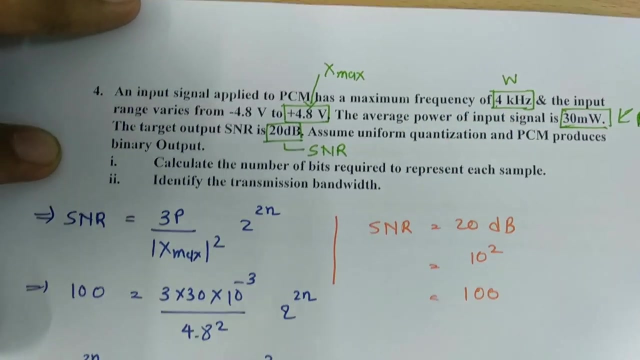 bandwidth, transmission bandwidth that i have already explained in last session. that will be number of bits into bandwidth of signal. number of bits is 8 and bandwidth of signal is 4 kilohertz. one can see here bandwidth of signal means maximum frequency in input signal. so bandwidth of signal. 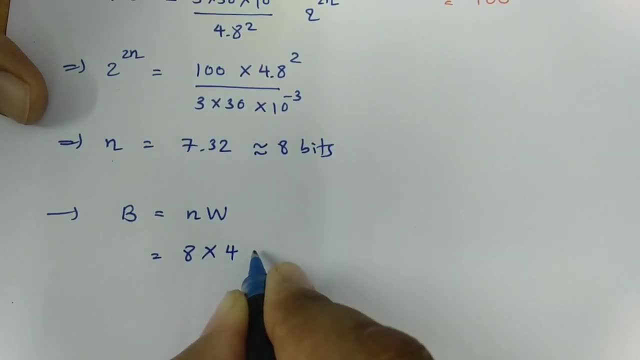 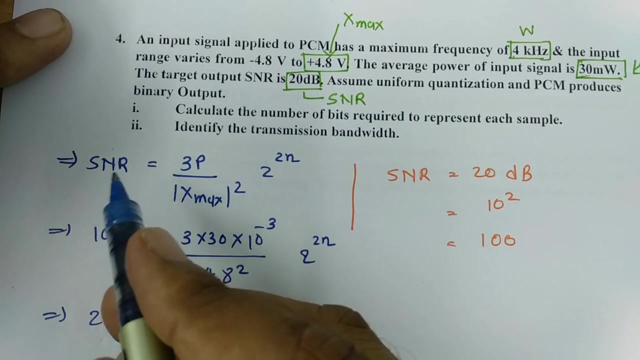 that is 4 kilohertz. so 8 into 4 kilohertz, so that will be 32 kilohertz. so bandwidth, transmission bandwidth, that will be 32 kilohertz. so here what is the difference? one should understand if input signal is not sinusoidal, in that case snr formula will be this: that will be 3p divided. 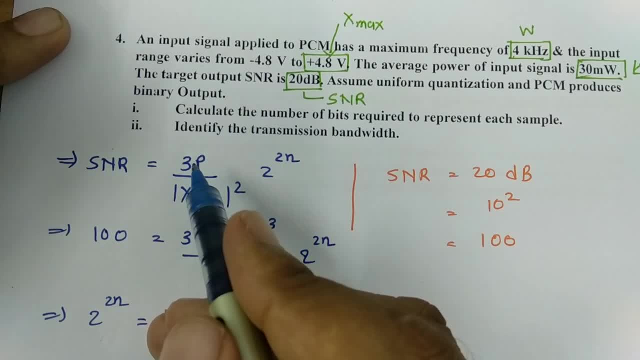 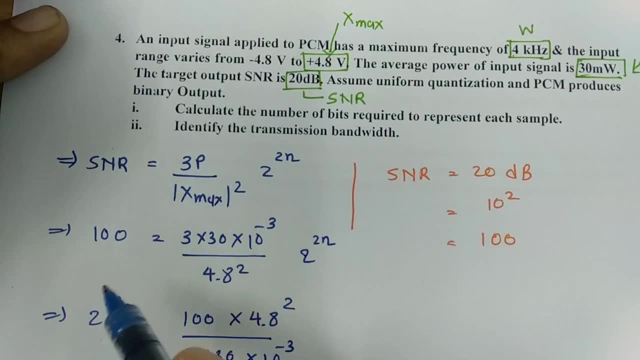 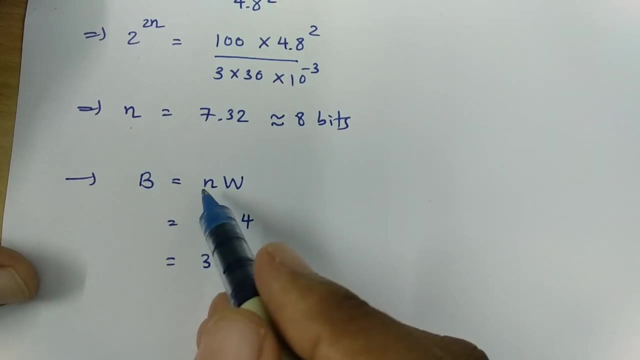 by x max, square into 2 to the power 2n, where p is power, x max is maximum amplitude and n is number of bits, and here other datas are given. we are delivered to calculate n. so that is what we are calculating by doing this calculation, and transmission bandwidth is number of bits into. 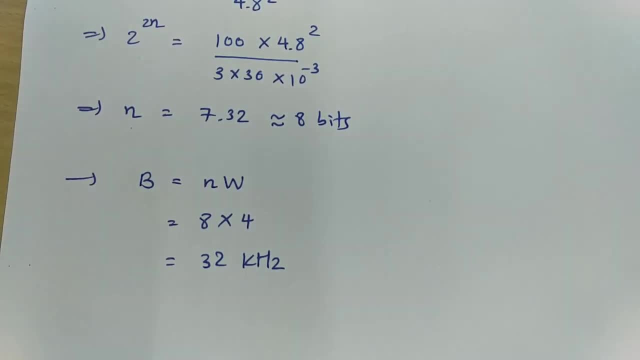 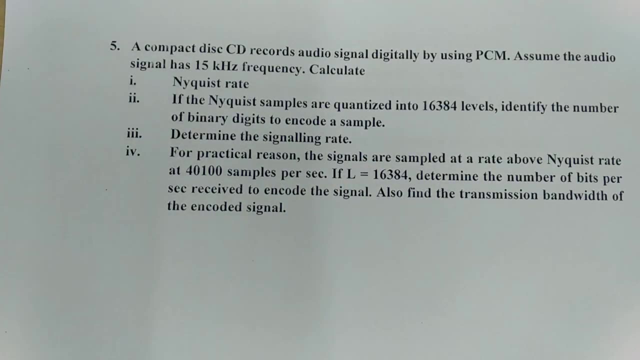 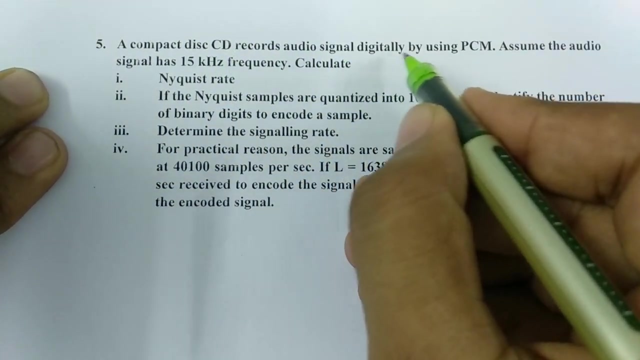 bandwidth of input signal. so that will be this. so this is how we can solve this problem. let us move on to next problem. so that will give little clear idea about pcm. now see a compact disc. cd records audio signal digitally by pcm. assume the audio signal has 15 kilohertz. so here: 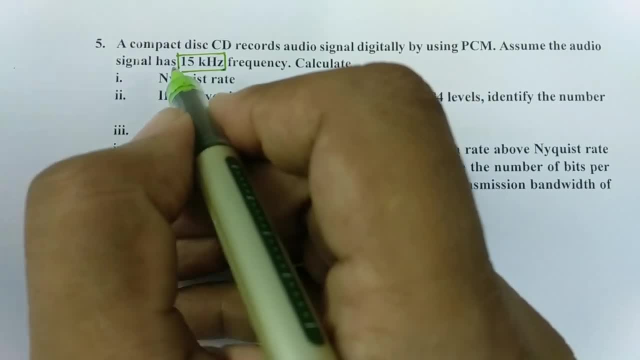 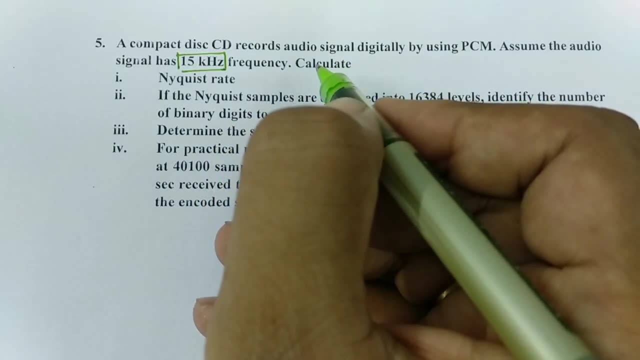 we have audio signal has 15 kilohertz. so here we have audio signal has 15 kilohertz. so here we have audio signal which is not sinusoidal signal. so if audio signal that is 15 kilohertz, that is not sinusoidal signal, calculate nyquist plot, nyquist rate sorry, and see this is what audio signal that. 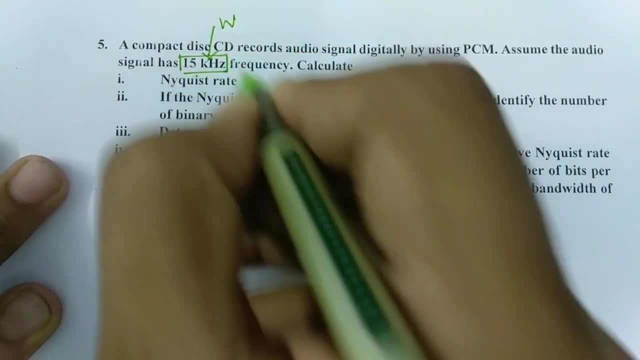 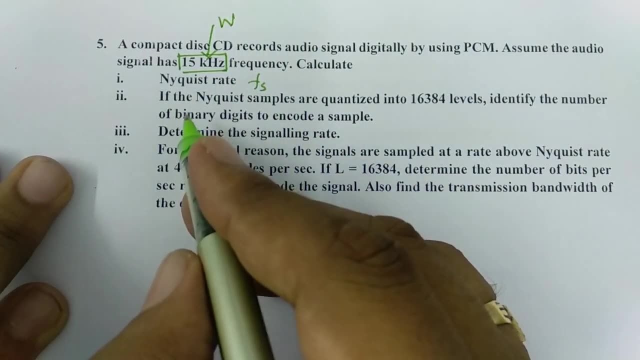 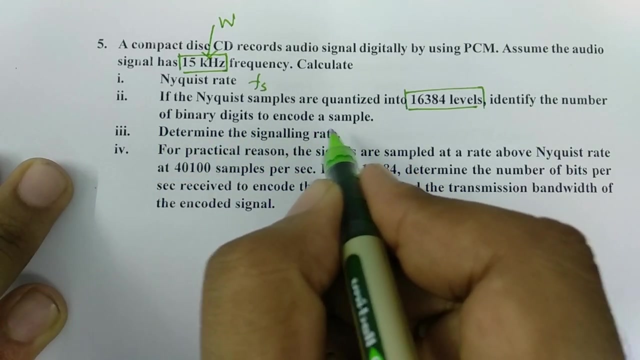 is having 15 kilohertz. frequency means its bandwidth. is this so nyquist rate, fs, that will be twice of the bandwidth of signal if nyquist samples are sampled at this many levels. identify binary digits. then third is determine sampling rate. so we are delivered to calculate bit. 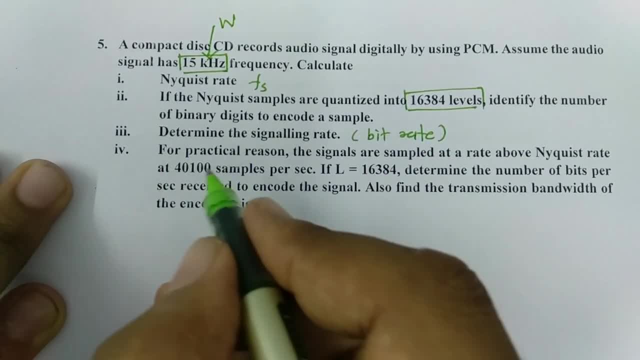 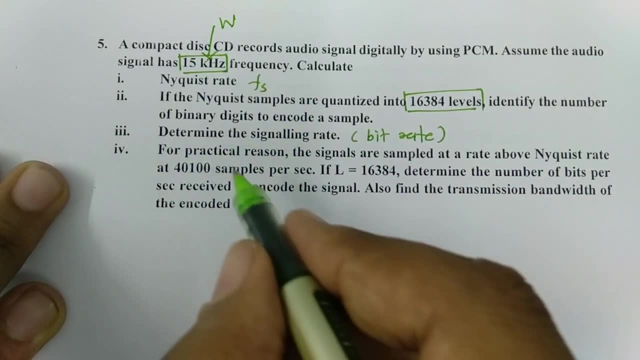 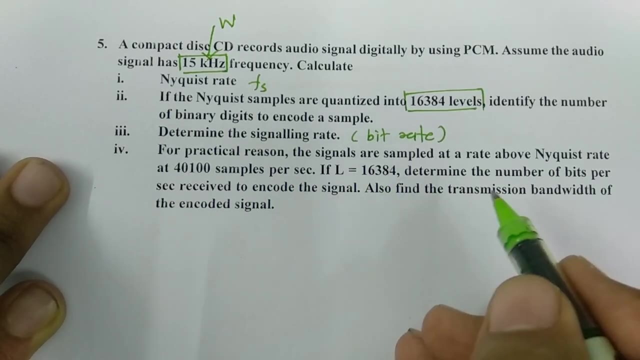 rate. and fourth is, for a practical reason, the signals are sampled at a rate above nyquist rate. so this is another case. so for that it's nyquist rate is this and l is this. in that case we are delivered to identify transmission bandwidth. so let us calculate one, two, three, four, five, six, seven. 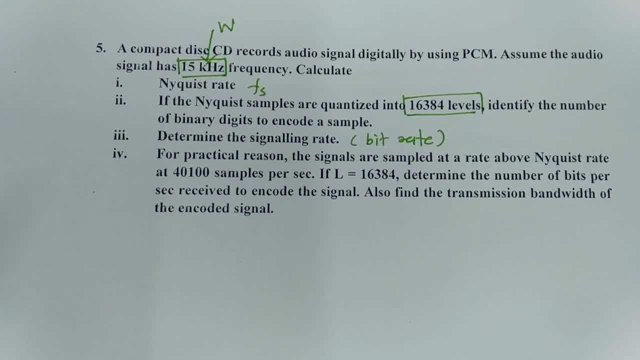 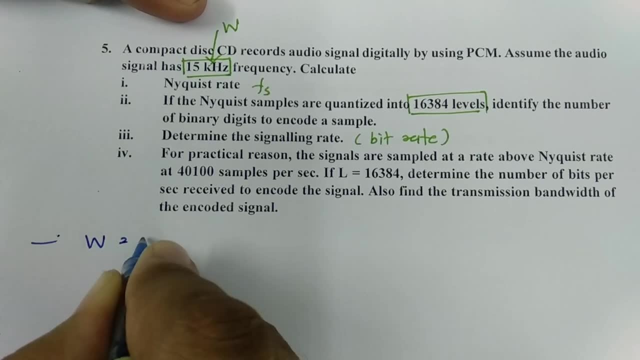 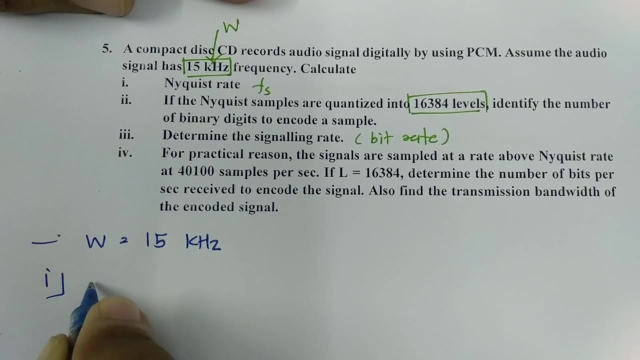 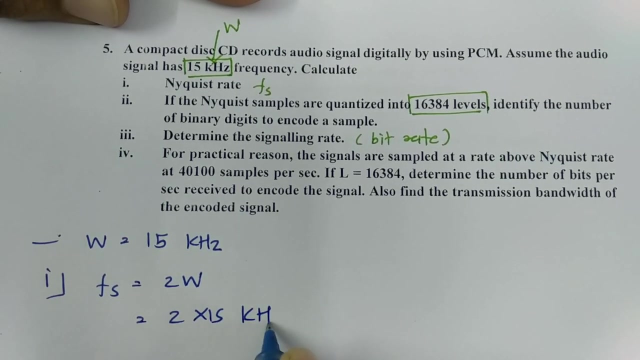 three first, and then we'll calculate fourth. so here, as i have told you, w is given, so w, that is 15 kilohertz. so from this we can calculate nyquist rate. so first nyquist rate, fs, that is twice of the bandwidth, so that is 2 into 15 kilohertz, so that will be 30 kilohertz. 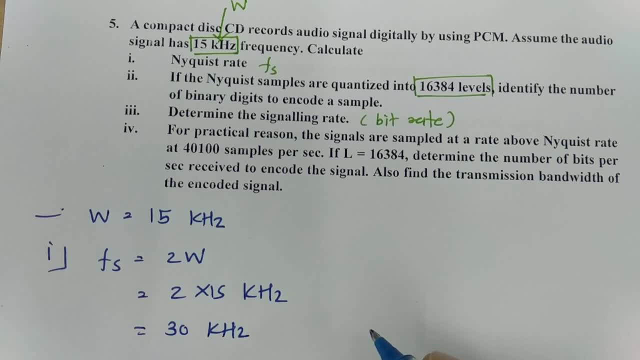 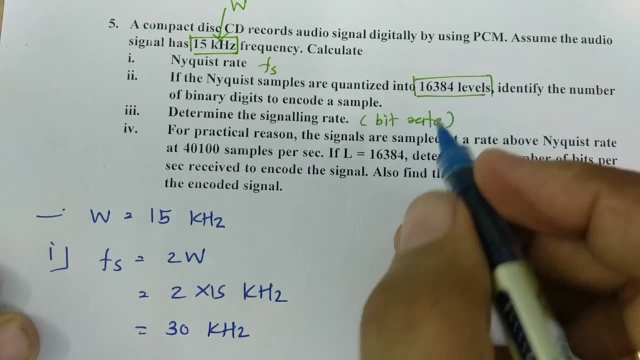 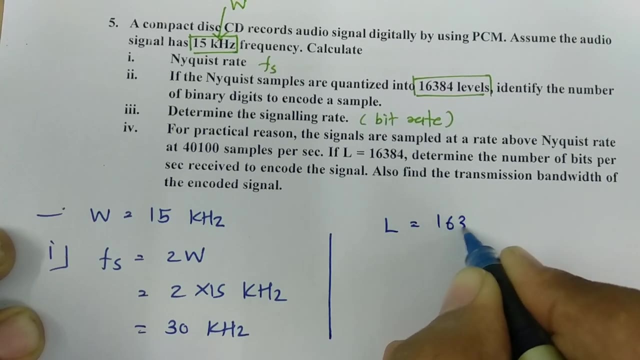 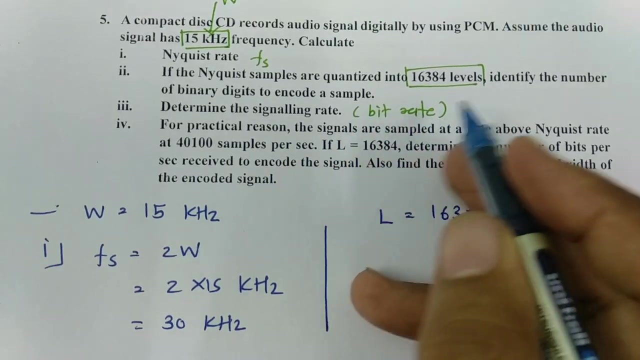 so nyquist rate is 30 kilohertz. now see second question is: l is given, number of levels, quantization levels, that is given. so if number of quantization level l is given, that is 16384. so in that case we are delivered to calculate number of bits. to identify a sample means. here we will be calculating. 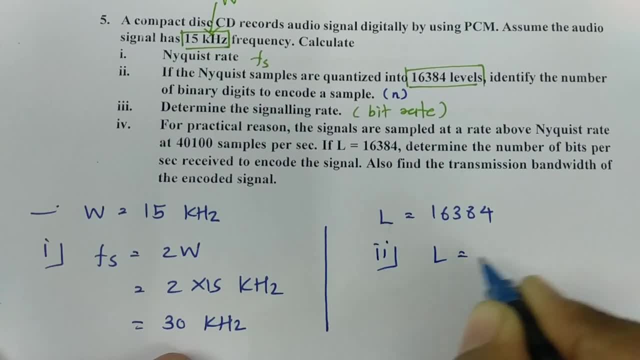 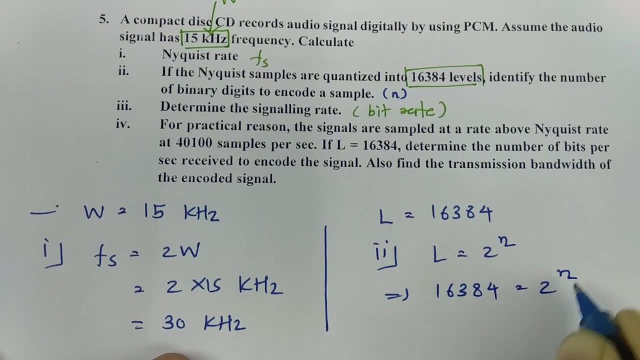 so, as we know, l is equals to 2 to the power n. so that is what: 6 16384 is equals to 2 to the power n. take log at both of the sides. so log 16384 is equals to n log of 2. so this is how we can have. 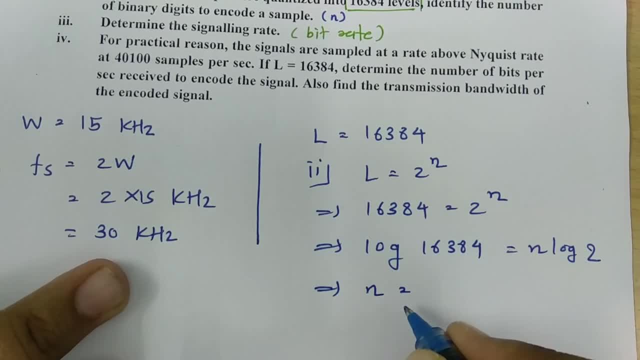 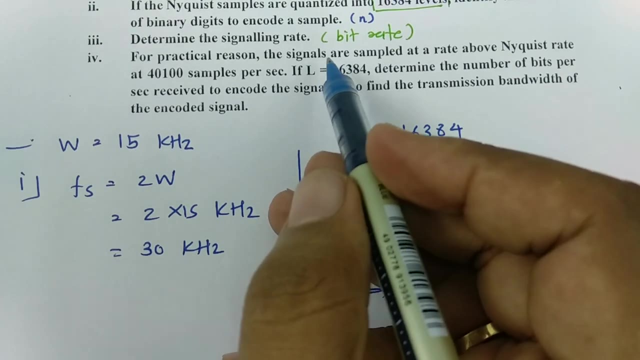 n. that is log of this divided by log of 2, and if you do this calculation, you will be getting n is equals to 14 bits. so now we have: n is equals to 14 bits as per this data. and third question, that is, what signaling rate? now see, as i have told you, signaling rate means bit rate and bit rate that is. 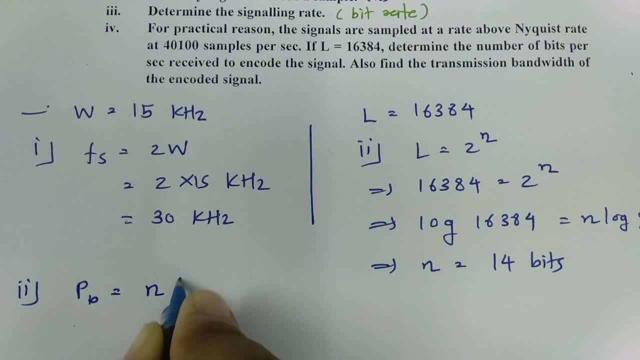 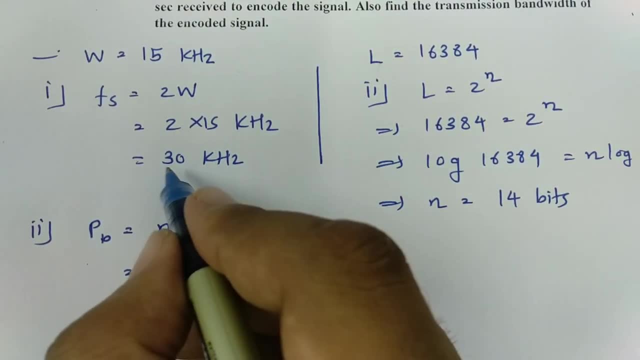 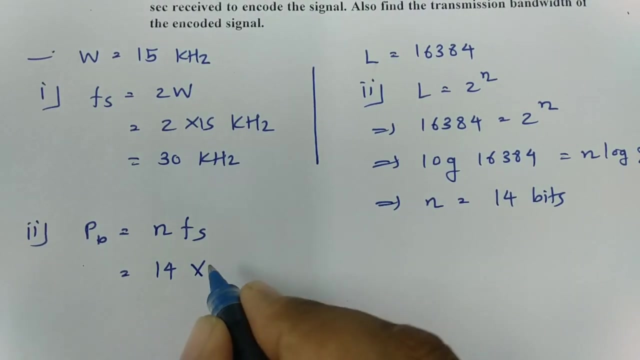 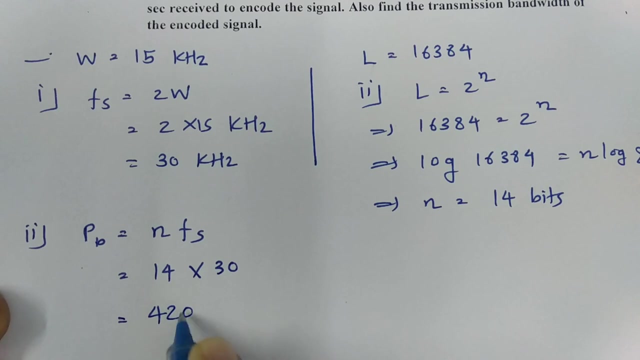 bit rate is pb and that is number of bits into sampling rate. so number of bits is 14 and sampling rate that is. we have calculated 30 kilohertz, so fs is 30 kilohertz. so if you place this 30 fs so you will be getting this is 420 and this is what 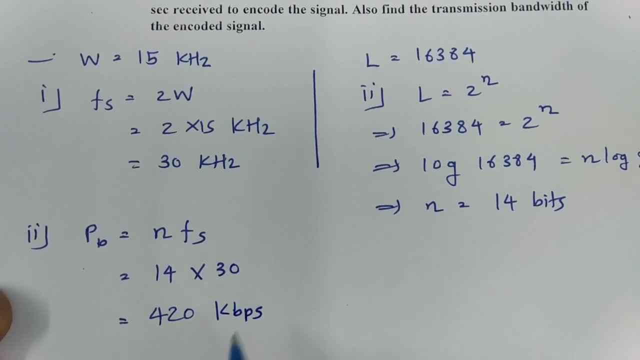 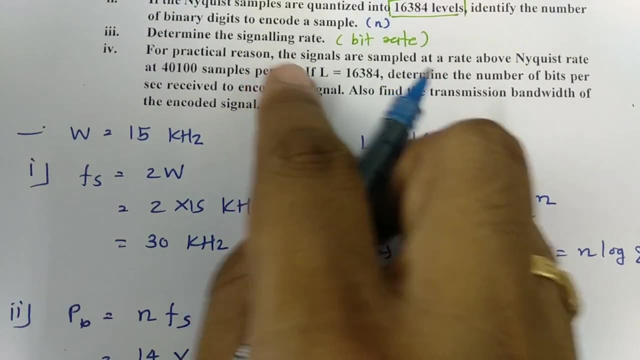 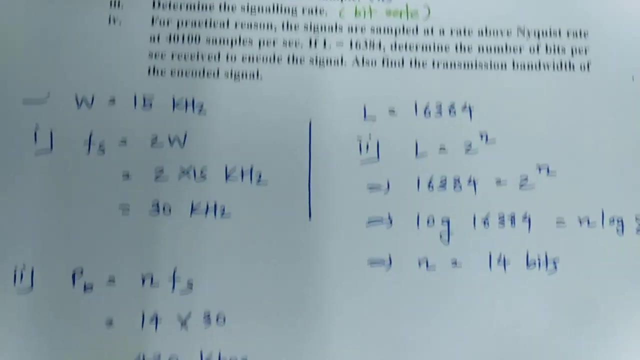 kilo. so that will be k b p s, so kilo bits per second. so this is what the case which will be over here now see. in fourth case, it is given nyquist rate is there at sample rate of four, one, four zero, double zero. so in fourth case, 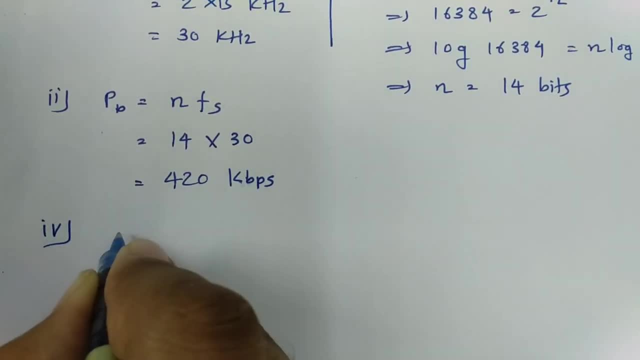 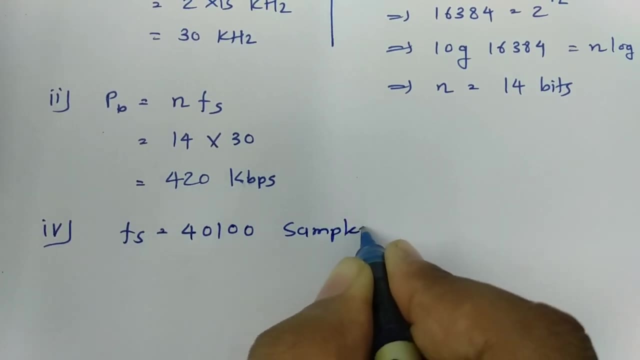 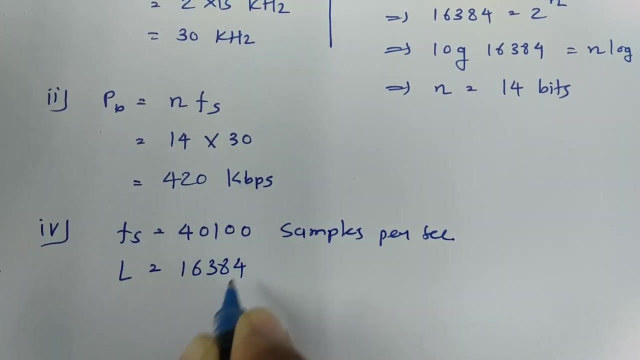 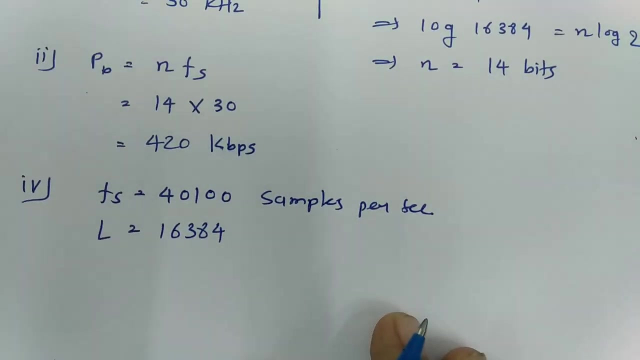 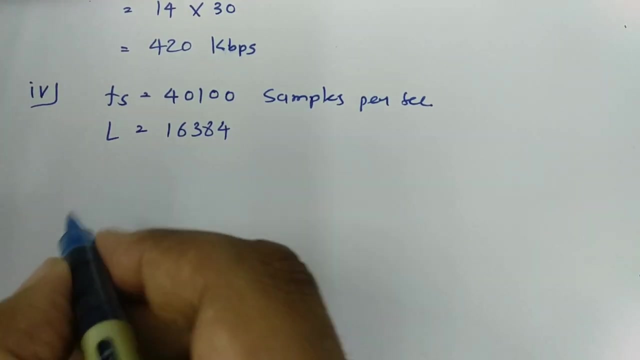 in fourth case, fs, that is given by 4, 0, one double zero samples per second, and l, that is given one, six, three, eight, four. you can see, l is even given. for this we are ready to calculate transmission bandwidth. so for transmission bandwidth, first we need to calculate n, and here we will be having n first, so n can be. 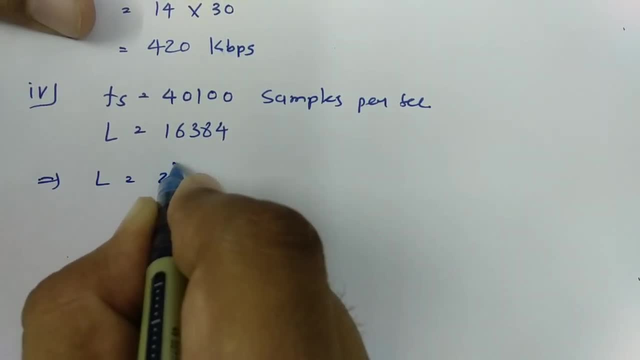 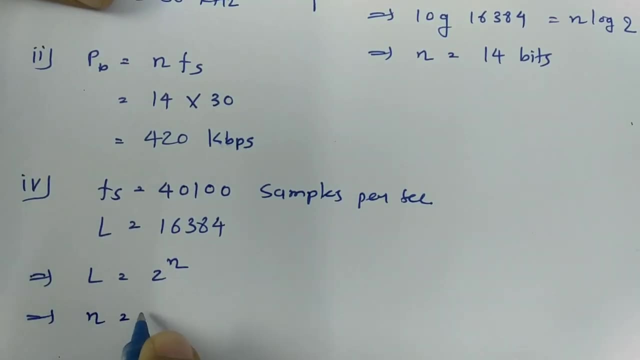 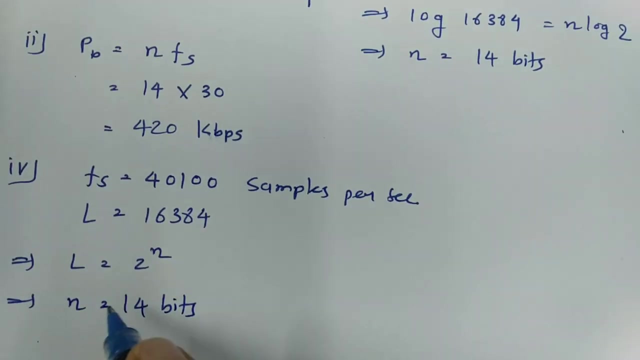 calculated as per l, l is equals to 2 to the power n, and this is what similar value. so we just directly place that. so n is equals to 14 bits. the reason is: l is same. so if you just calculate as per this calculation, you will be getting n is equals to 14 bits. so one data that you have now. 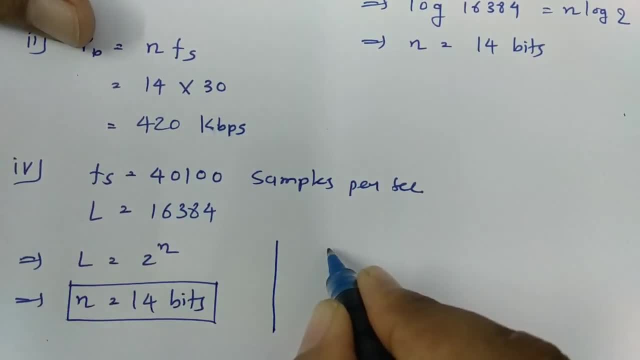 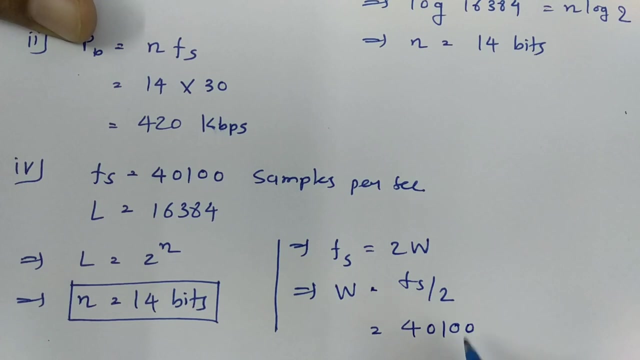 and now to have a w, you can have sampling rate that is twice of the bandwidth, so bandwidth of message signal that one can have. so that is fs by 2 and that will be 4: 0, 1 double 0 by 2, so that will result into: 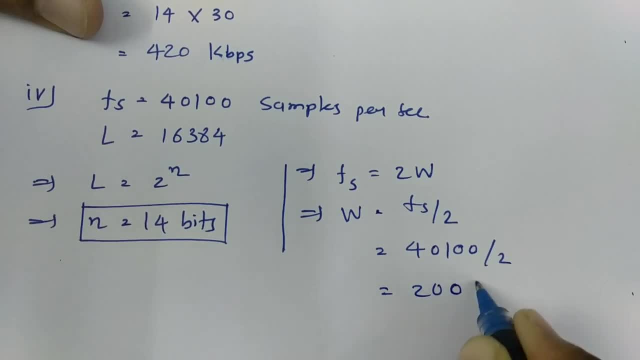 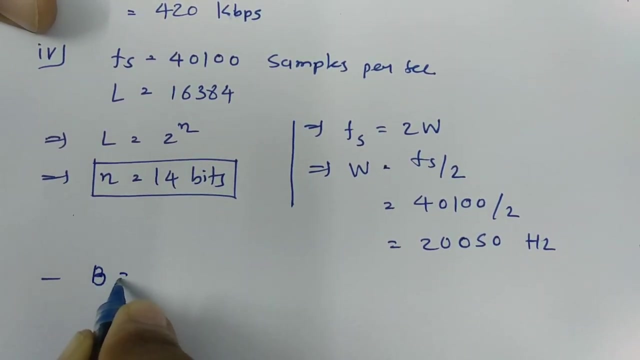 2 0 0, 5 2 0 0, 5. 2 0 0, 5 0. now we have this bandwidth, so we can have transmission bandwidth now and transmission bandwidth that, as we know, transmission bandwidth is n into w, so n is 14 into w. that is this. 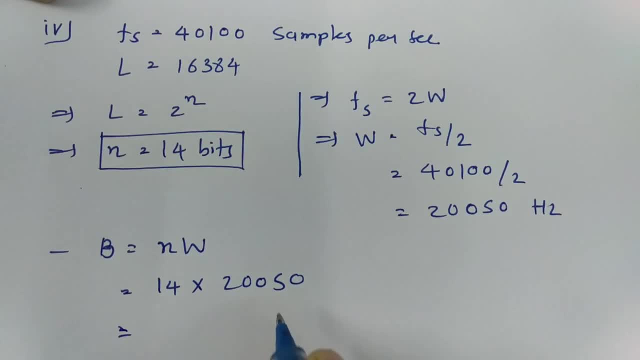 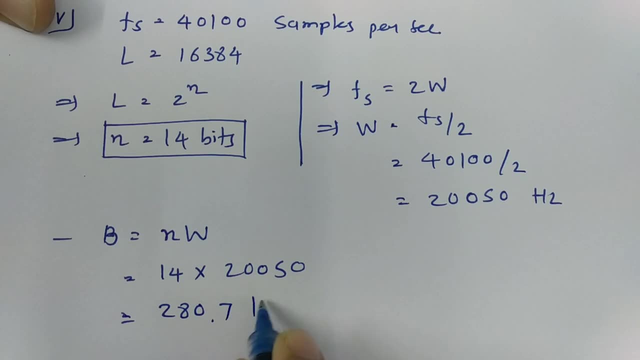 2 double 0, 5, 0, so you will be getting transmission bandwidth. that is, if you calculate this, you will be getting. it will be 280.7, 0.37, 0.37 kilo hertz. so this is what transmission bandwidth. 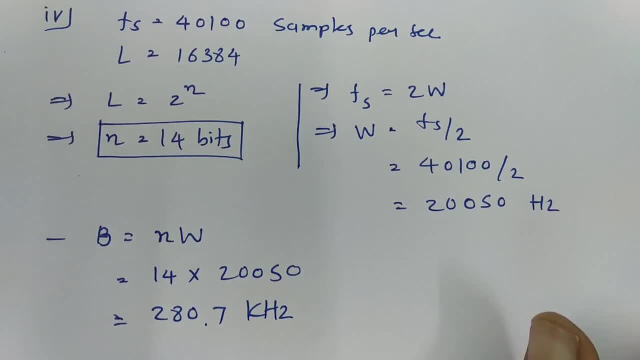 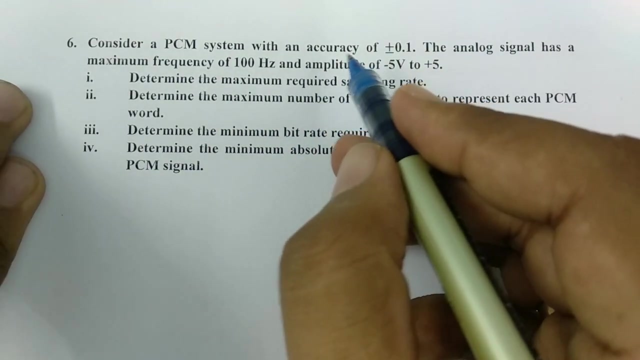 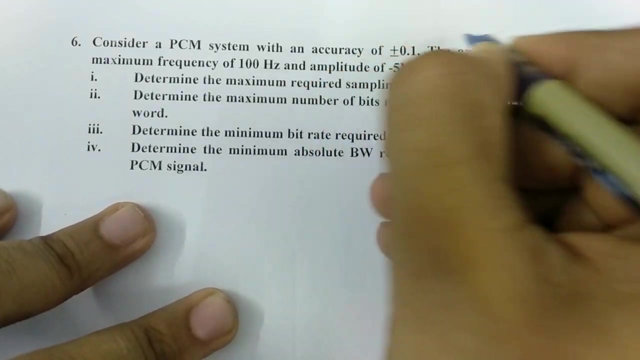 now let us have one more problem. so this will gives you little more clear idea about ccm pulse code modulation. so here in this question we have accuracy of quantization. so what is accuracy? accuracy of quantization so that we know for mid rise as well as mid trade. 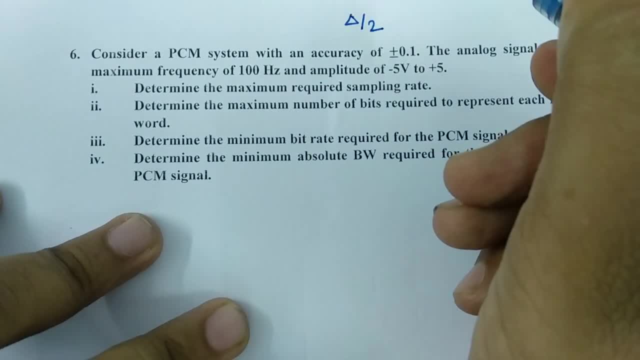 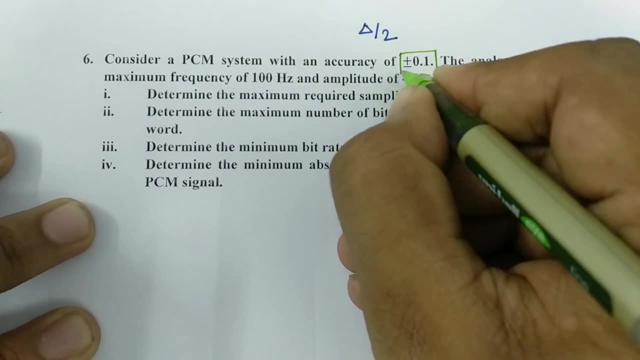 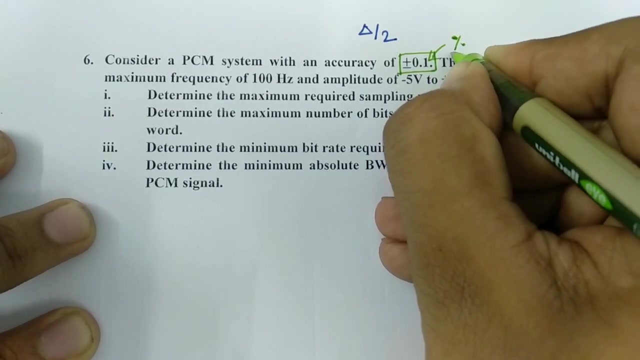 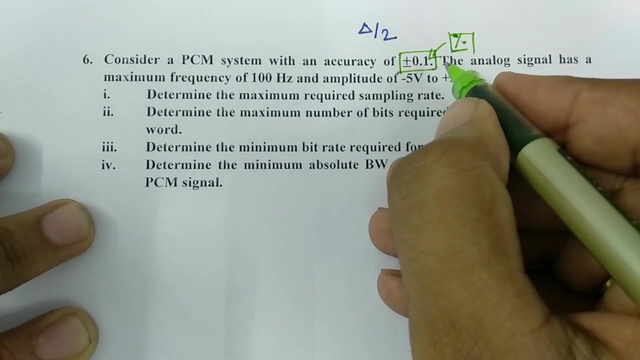 accuracy of quantization is delta by 2. so here accuracy is given 0. plus or minus 0.1, and here it is given in terms of percentage. actually, i forgot to mention that in this question it is given in terms of percentage. remember this. this is what plus or minus 0.1 percentage? if it is not given in terms of. 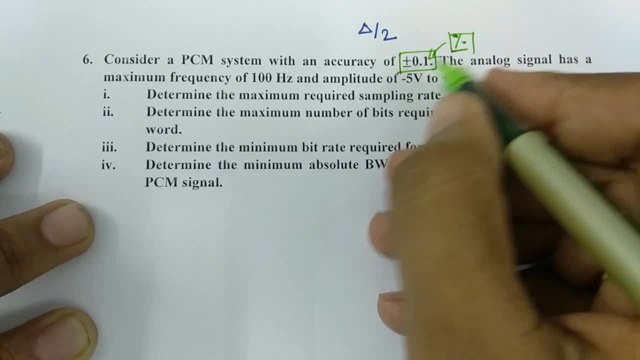 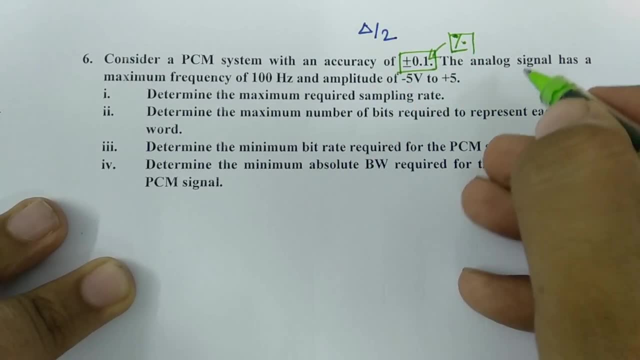 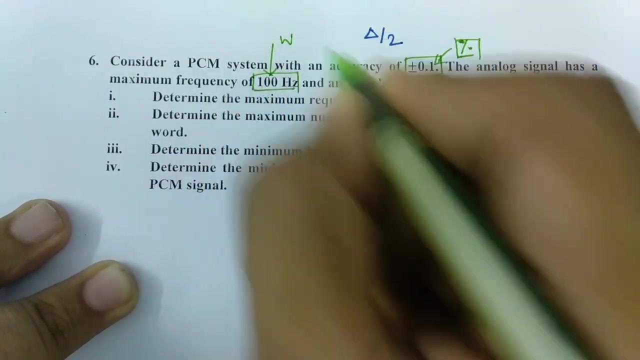 percentage. you should calculate it, but here it is given, so i'm just mentioning it. it is given in terms of percentage i'm mentioning here, and that accuracy is what: delta by 2 the analog signal has maximum frequency 100 hertz. so here one more thing that is given, that is w and amplitude varies. 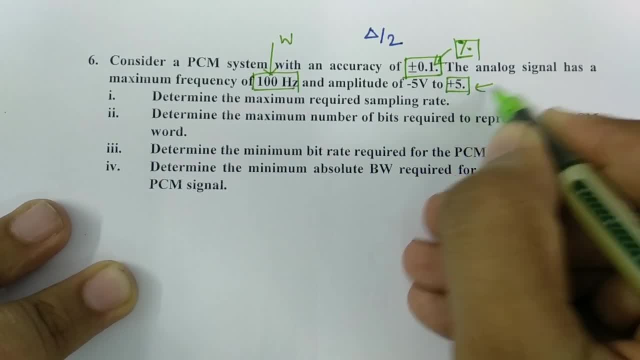 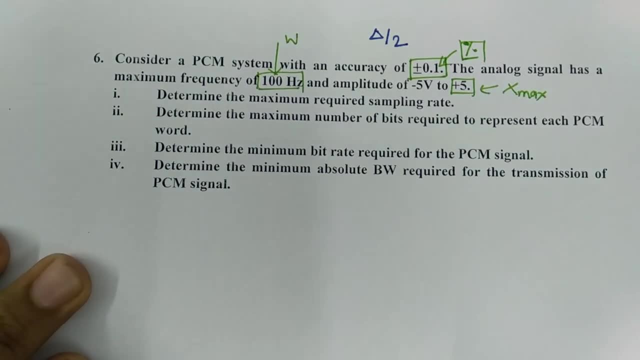 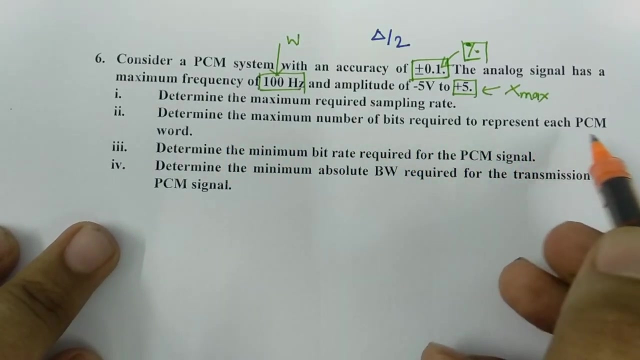 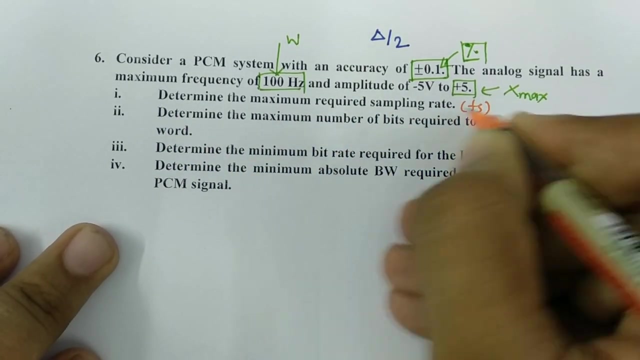 from minus 5 to plus 5. so x max 1, given that is what 5. so we are delivered to calculate 0.1 maximum required sampling rate. determine the maximum number of bits required to represent pcm word. so ultimately, here we need to calculate fs, here we need to calculate number of bits. 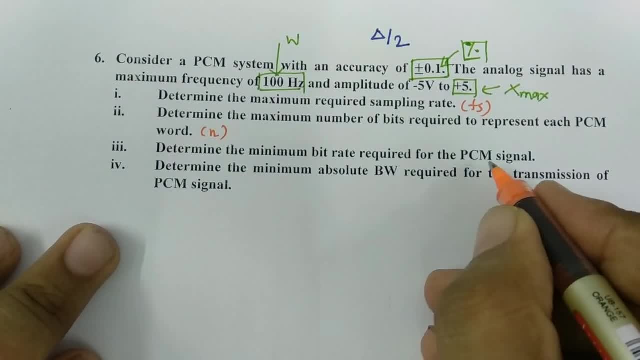 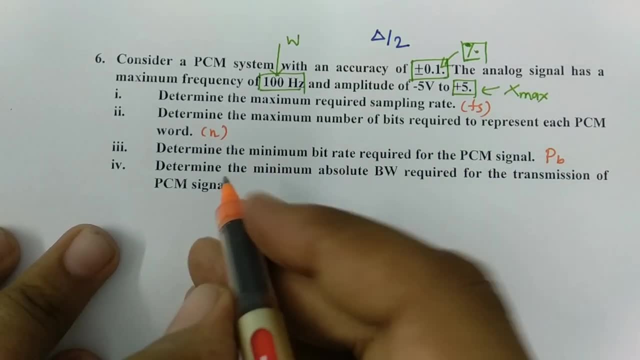 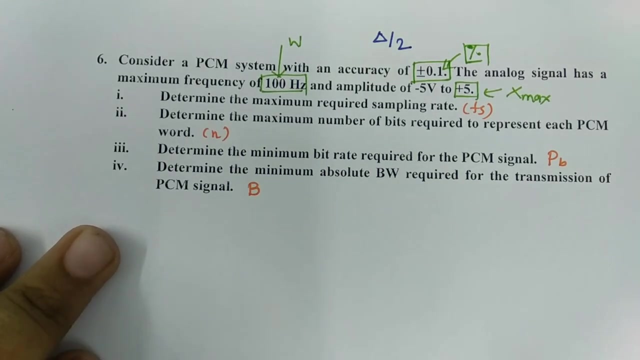 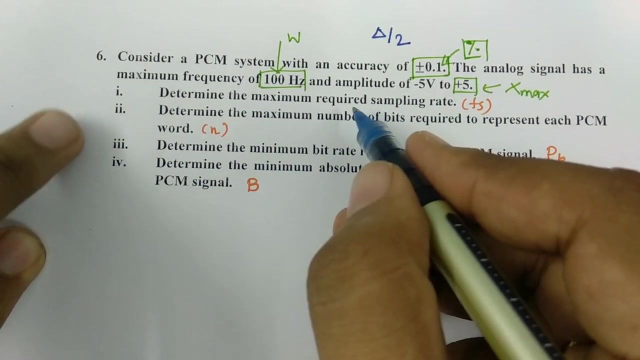 determine the minimum bit rate required for pcm signal. so here we are delivered to calculate bit rate pb and here determine the minimum absolute bandwidth required to transmit pcm signal. so here we are delivered to calculate bandwidth. so this many things that we need to calculate here. so see here first: that is what sampling rate and that we can easily. 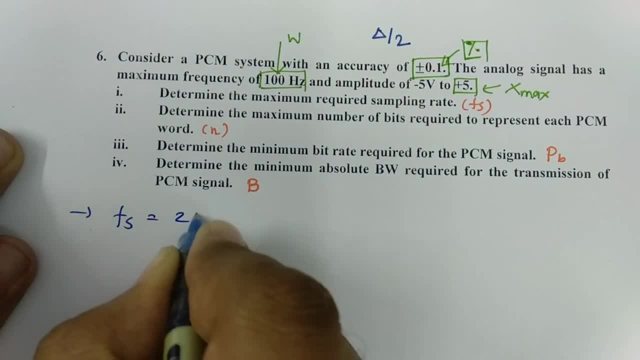 calculate sampling rate. that is twice of the bandwidth and that is 2 into. bandwidth is 100, so it will be 200 hertz. so sampling rate, that is what twice of the bandwidth of message signal. now, second is that this is what pcm signal command two, that is, pb and pcm signal. 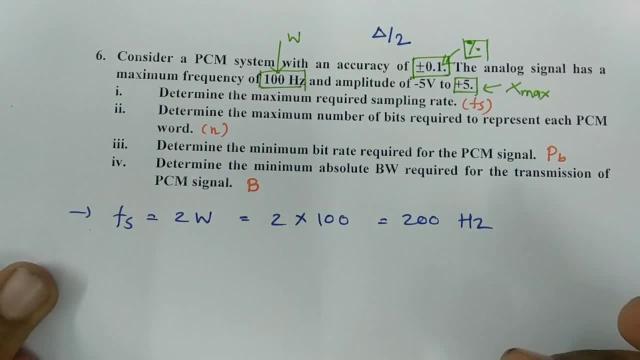 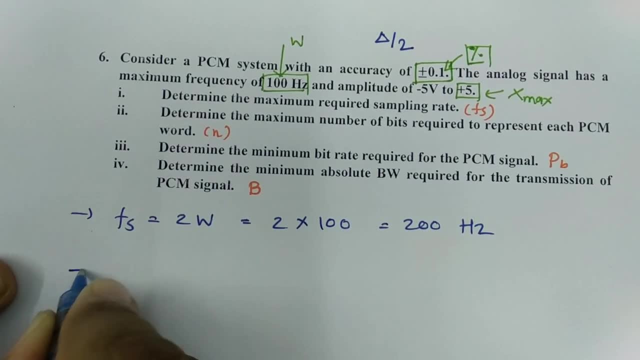 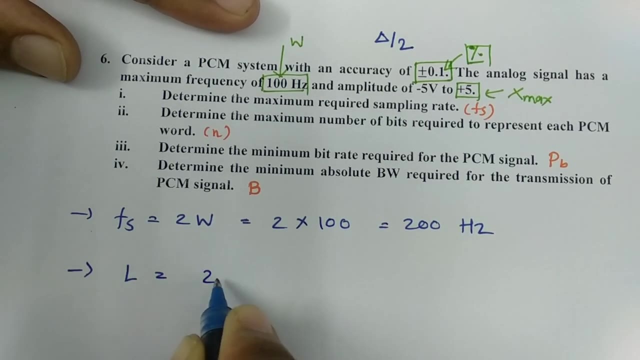 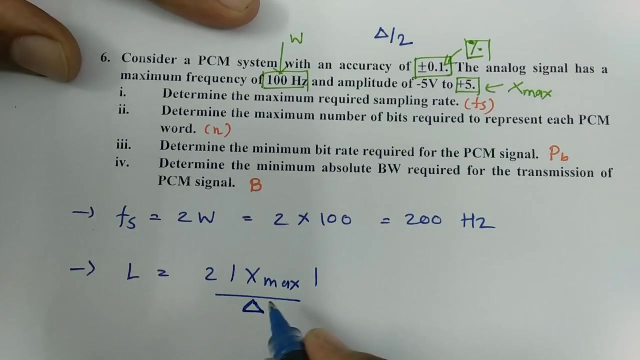 is determine the maximum number of bits required to represent that. now for that. this is not actually sinusoidal signal. so basic formula, basic formula of this will be: length. L is equals to 2 into X max divided by Delta. now here we need to calculate L and from L will: 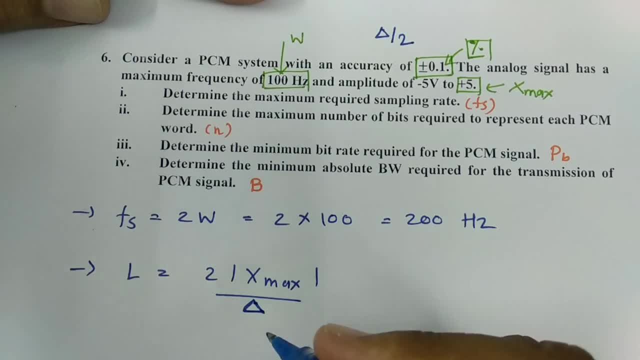 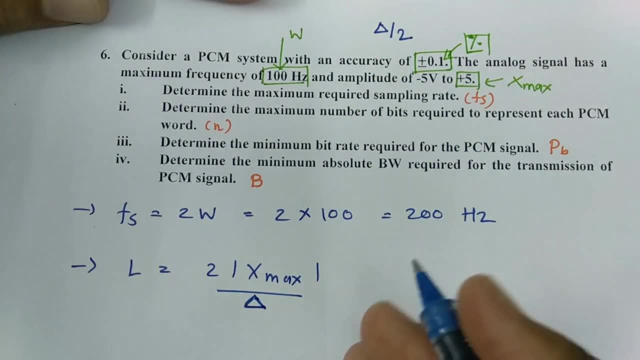 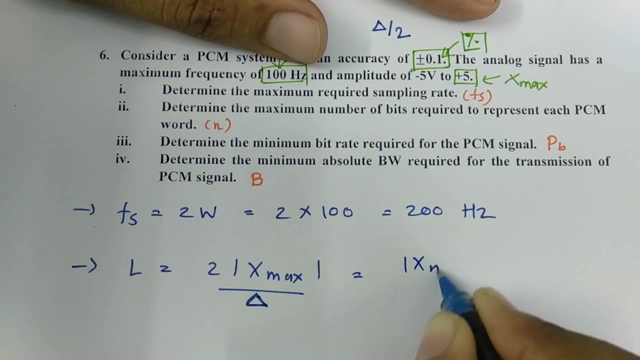 be calculating. and now here, Delta, that is the question. now, see Delta, that is what already given accuracy, that is what 0.1 percentage? so Delta by 2, that is 0.1 percentage. so actually I am just writing this over here like see X max, that is X max by Delta by 2. okay, so, 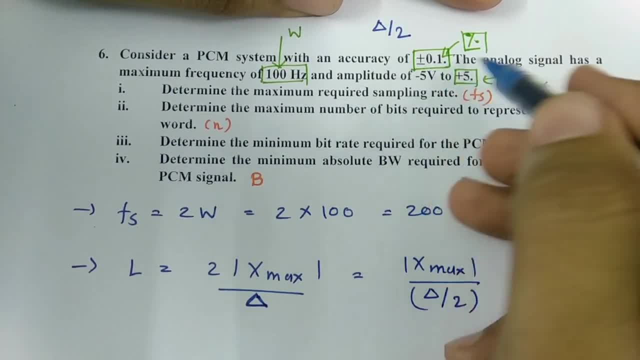 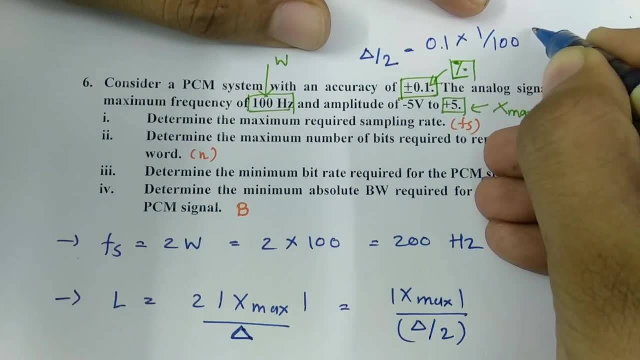 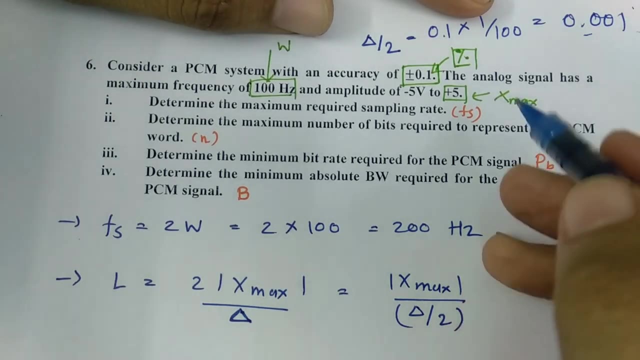 Delta by 2, that is what accuracy of PCM that is. 0.1 percentage, it means it is 0.1 percentage. 1 into 1 by 100, it means it will be 0.001. so Delta by 2, that will be 0.001 and X max. 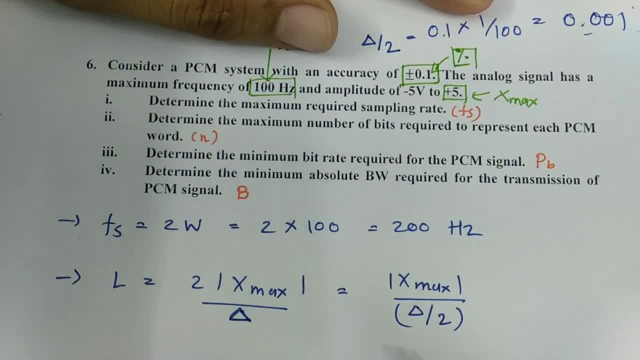 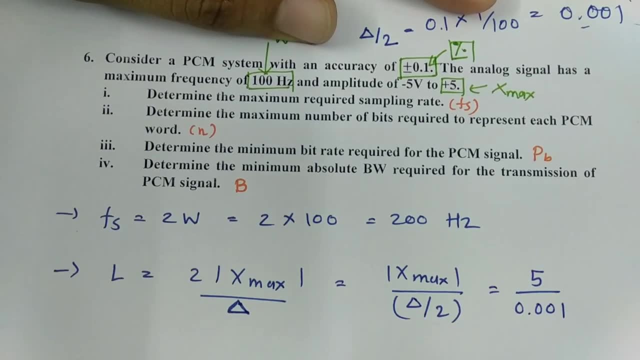 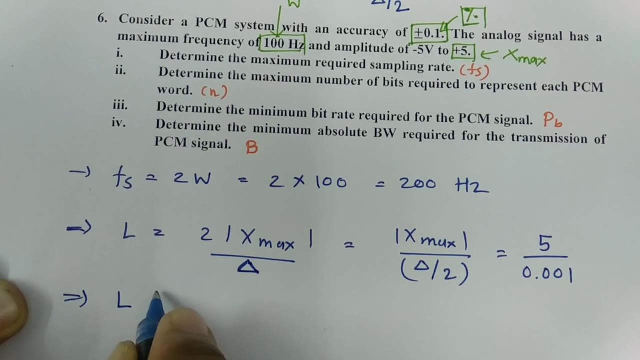 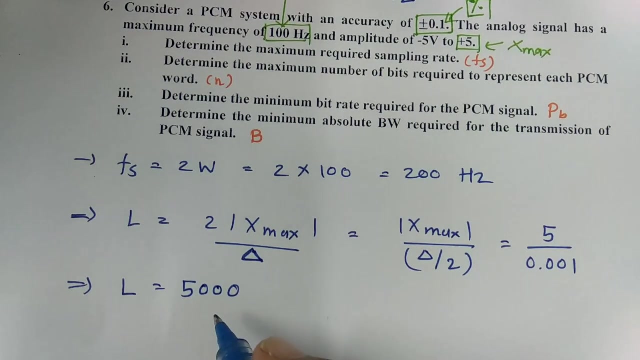 that is 5 and L that we can identify from it. so X max, that is 5 divided by 0.001. just calculate this so you will be getting L and that is 5000. now, once you have L is equals to 5000. from this you can calculate n. so L is 2 to. 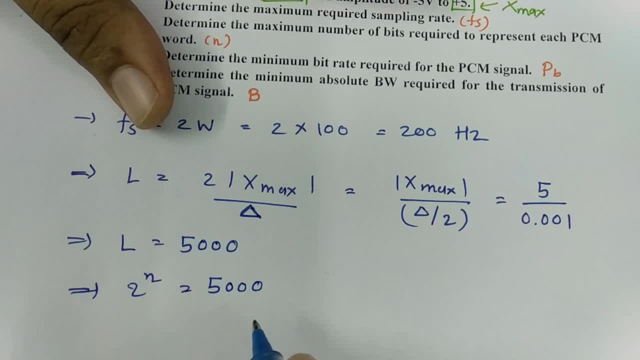 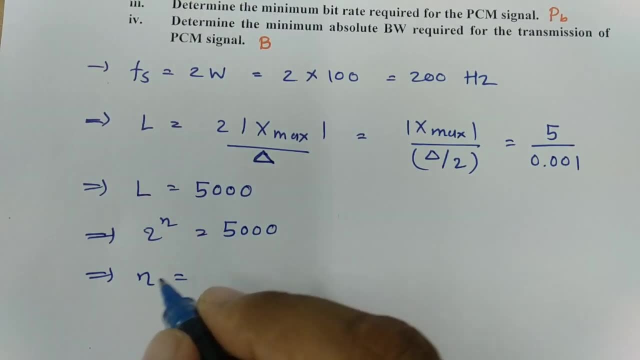 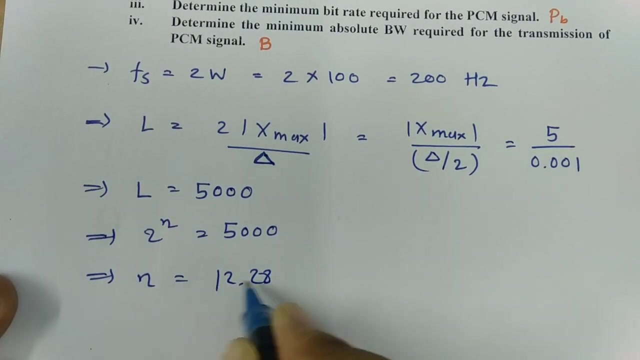 the power n, that is equals to 5000. take log at both of the side. you will be getting n here. I am not calculating it. log of 5000 divided by log of 2, that is n, and you will be getting. this will be 12.28 and you cannot take in this form. so you will have to have. 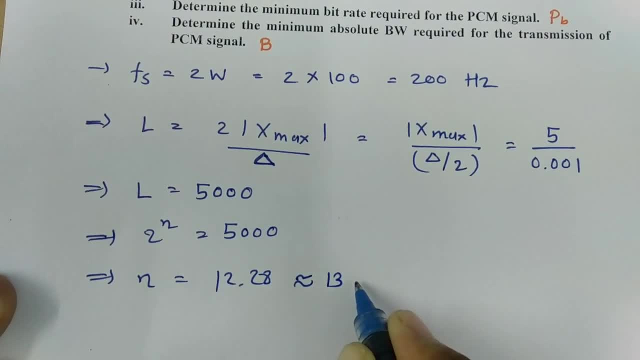 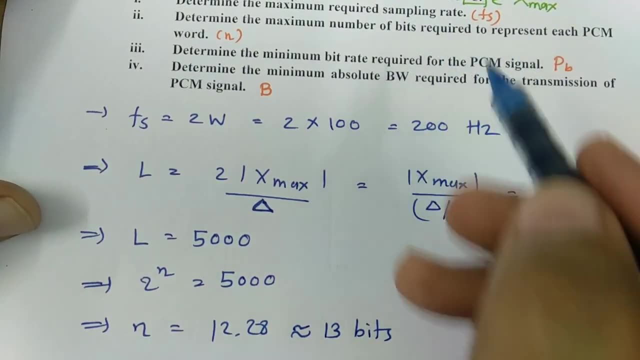 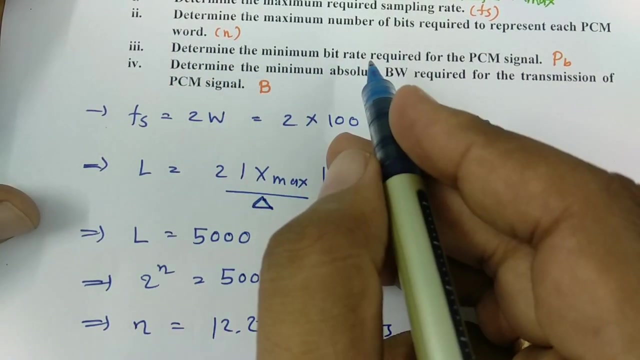 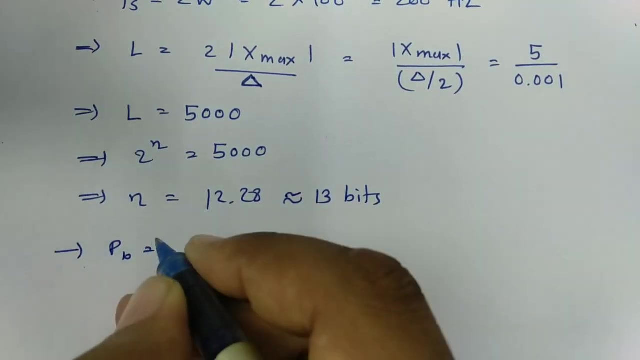 greater than this round off. so it will be 13 bits. so number of bits required, minimum number of bits: that is 13 bits, which is required over here. so n is equals to 13. now, third case: that is what determine the bit rate of this? so bit rate Pb, bit rate Pb, that is number. 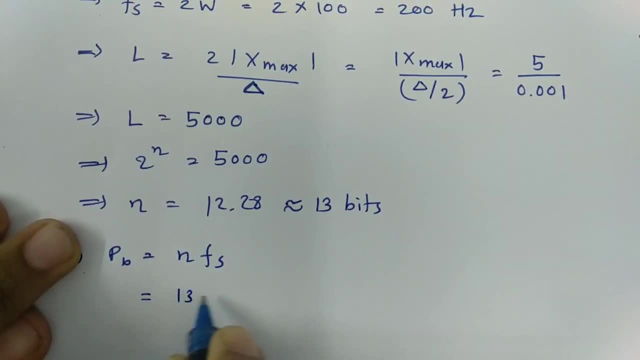 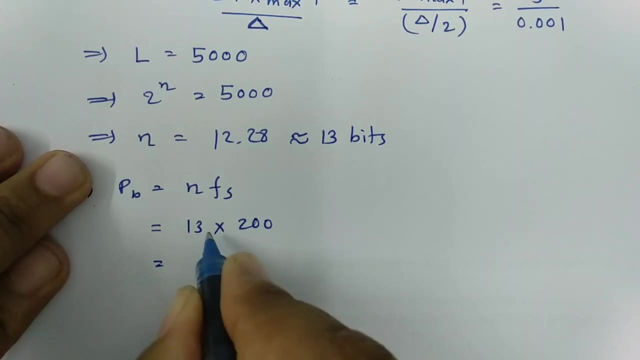 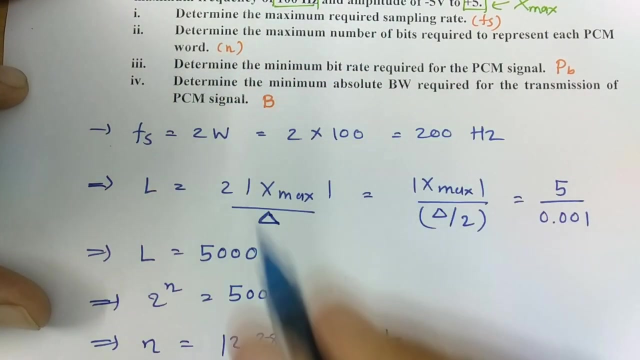 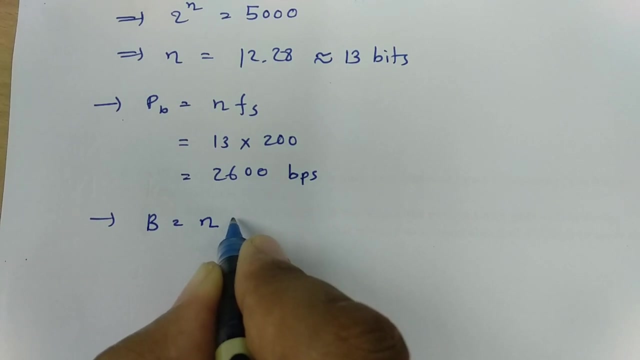